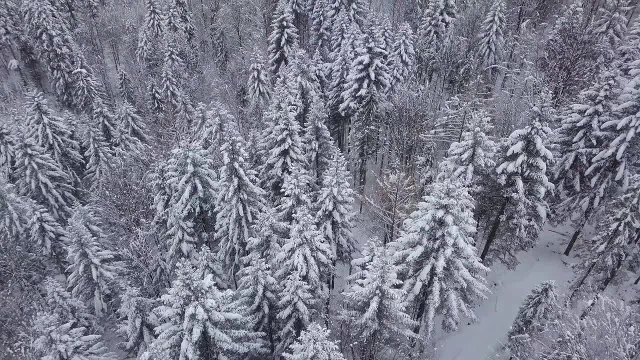 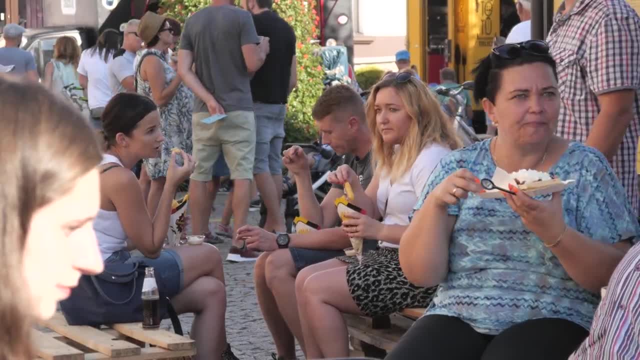 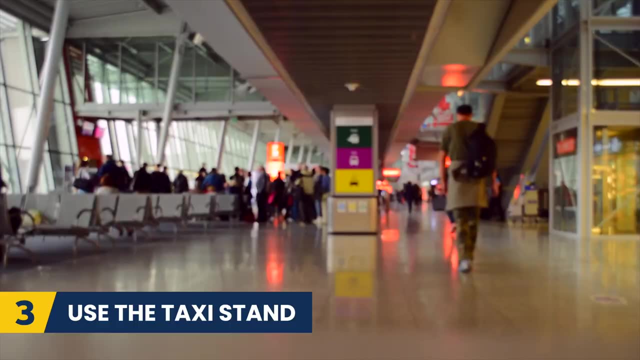 winter, so it's best to avoid this time if you can. Summer in Poland is glorious and you can visit at this time, but expect higher hotel rooms and the crowds. So the next thing you need to know before you go to Poland is to use the taxi stands As you arrive at any of the major airports in Poland. there are 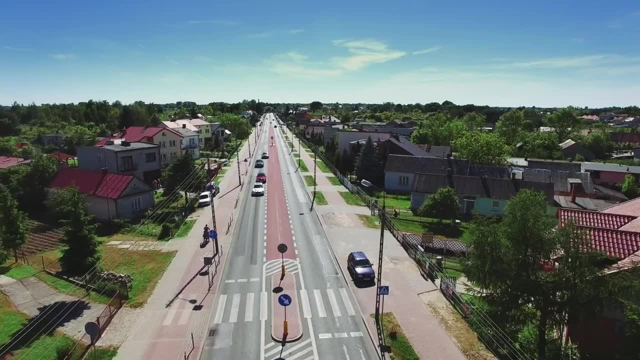 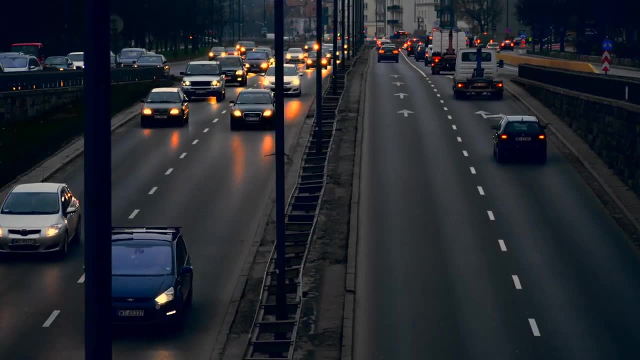 designated taxi stands at the airports. Make sure to use these and avoid the drivers who approach tourists in the arrivals terminal. Only official taxi drivers will run the meter, so make sure to carry a proof of medical insurance before you go to Poland. If you have a, 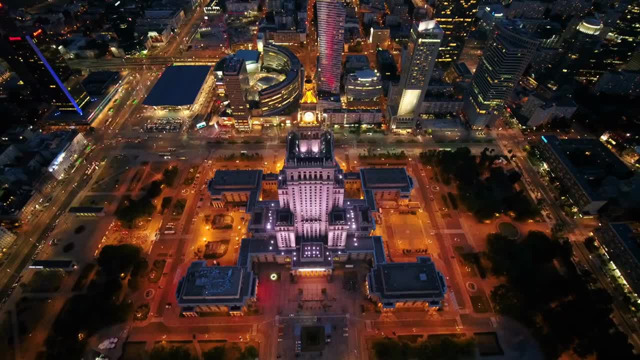 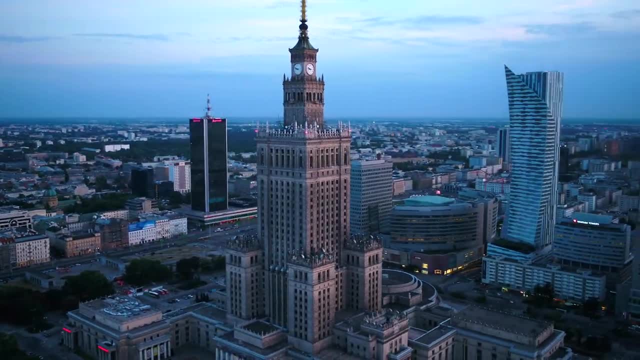 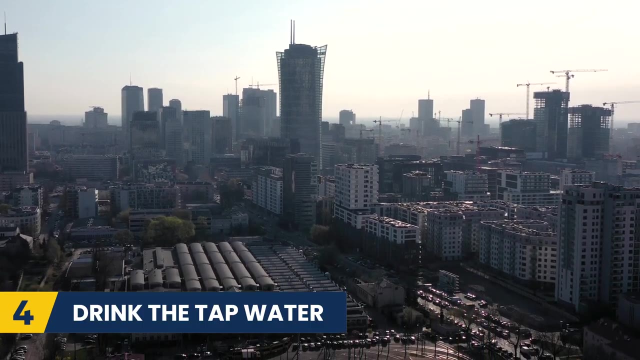 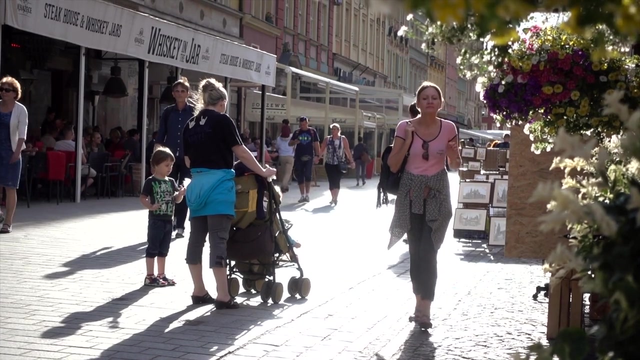 visa, you will need to carry small notes to pay the correct fare. Another thing to know before you go is that tap water is safe to drink. Following EU regulations, tap water is safe to drink in Poland. However, the older generation don't quite believe this yet, so ordering tap water in restaurants. 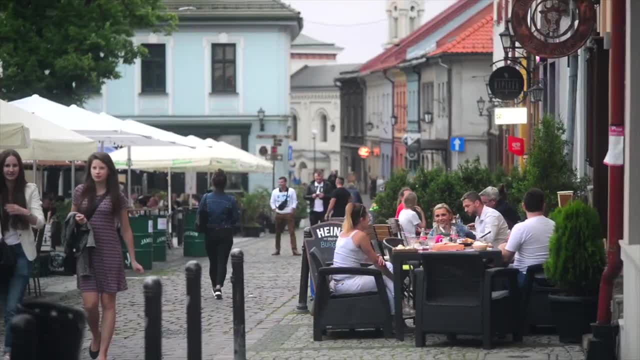 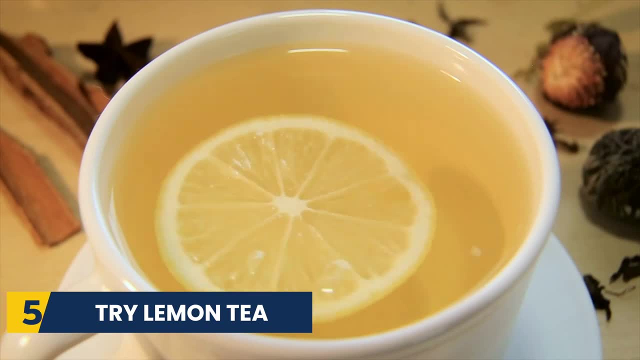 may still get you a few weird looks. And whilst we are talking about drinking in Poland, why not try some lemon tea? When ordering a cup of tea in Poland, don't expect to have milk with it. Instead, you could ask for a slice of lemon trying it. 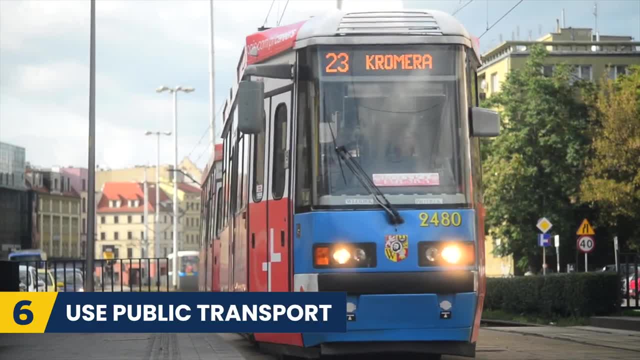 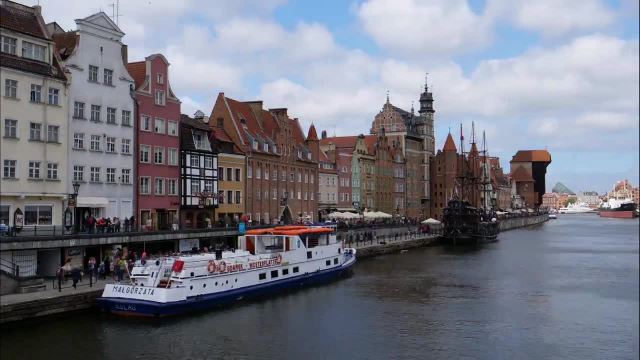 the Polish way. Another thing to know is to use public transport. Getting around Poland is super easy. The country, although large, has an excellent train and bus network, so that you can drive around Poland easily. The country, although large, has an excellent train and bus network so that you can drive around it拝. 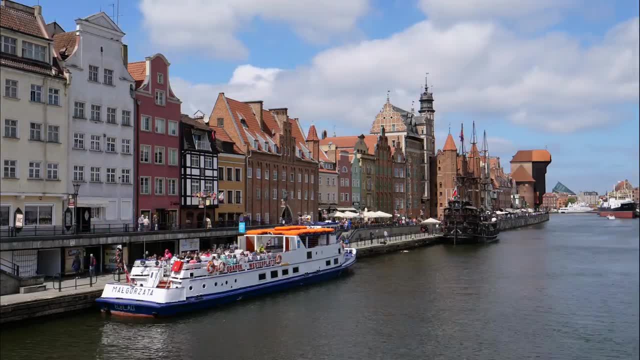 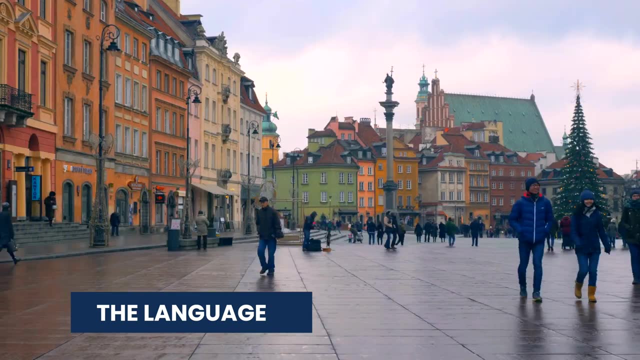 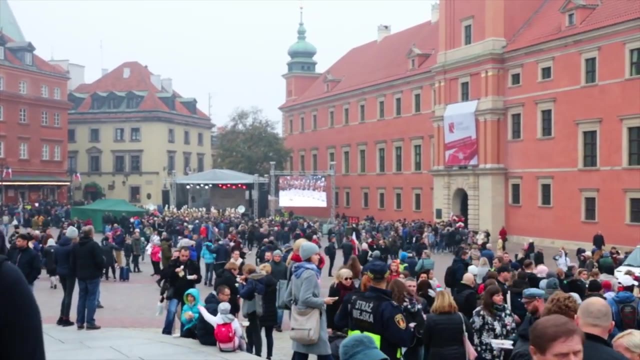 so that you can transfer from one city to another with ease. Let's quickly talk about the language for a second. So the Polish language is tricky to learn, but try to learn some basic phrases. You may get a few giggles from locals when trying to use it, but do not be offended. Making fun of 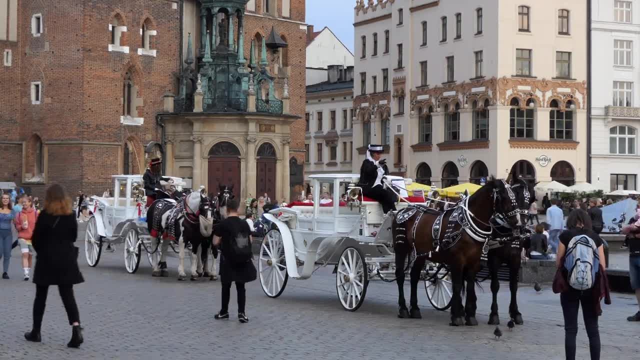 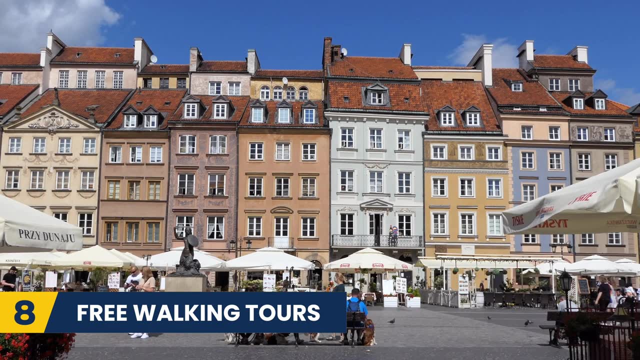 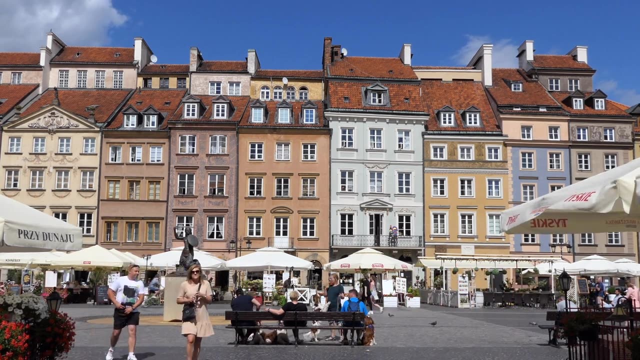 others is a sign of friendship in Poland. Another great thing about Poland is that there are plenty of free walking tours. In every major city there are free walking tours that you can take to save money and see the sights. And talking about saving money, Poland is one of the cheapest places to